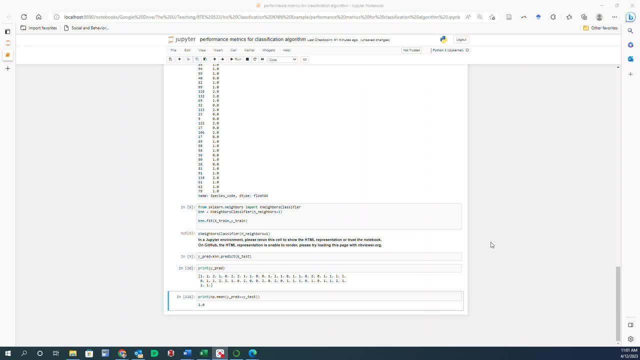 So, as an example, I'm going to continue working off of the file that we have been working on about the classification of iris species into three classes. So I will put a link to the video on which I went through all of this and I'm going to just continue working based on that. 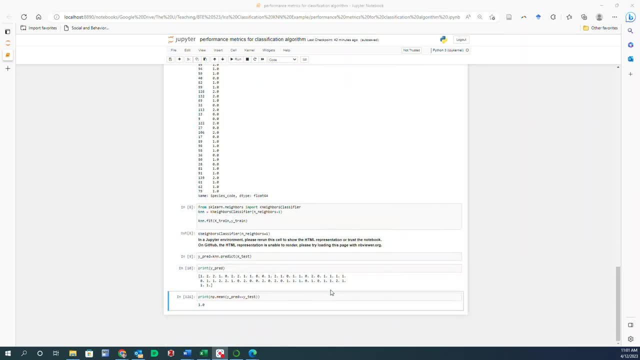 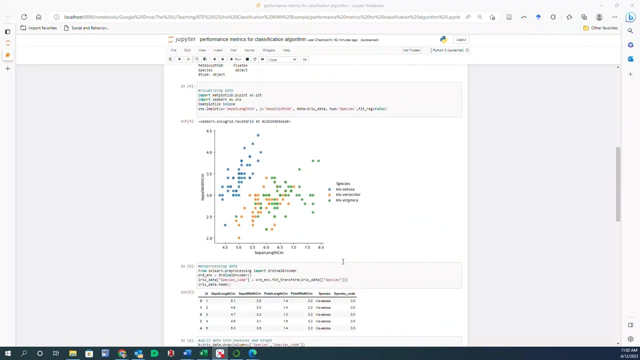 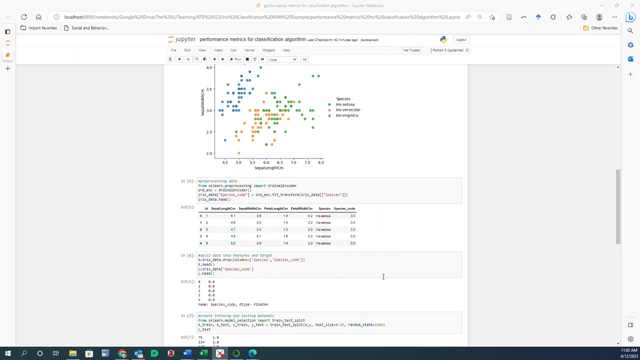 So far, what we have done is that we've implemented a k-nearest neighbor algorithm in order to classify different species, This different species of iris, into three groups, which were basically Satosa, Versicolor and Virginica- And note that here the KNN did especially good, meaning that they're 100% accuracy. 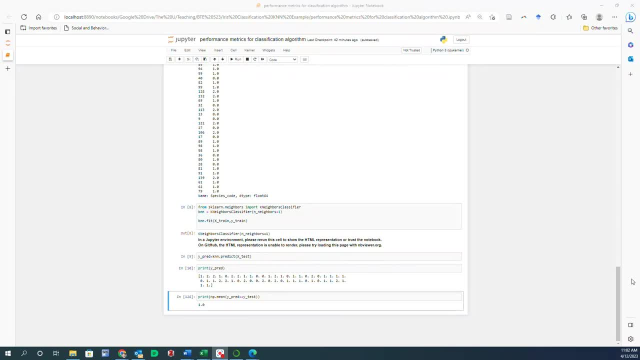 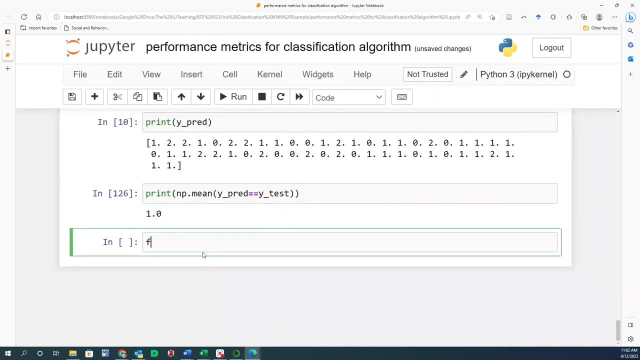 Anyways, I'm going to create two things. First, I'm going to create a confusion matrix, and then I'm also going to create a performance report for the algorithm. And to do that, the very first thing that you have to do is to import metrics from sklearn. So I'm going to insert a cell below and go ahead and type in from sklearnmetrics. import from sklearn. 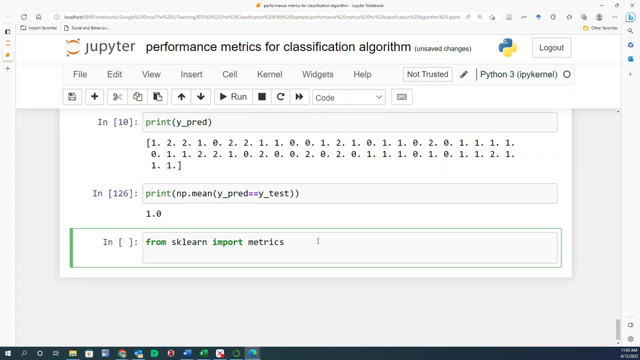 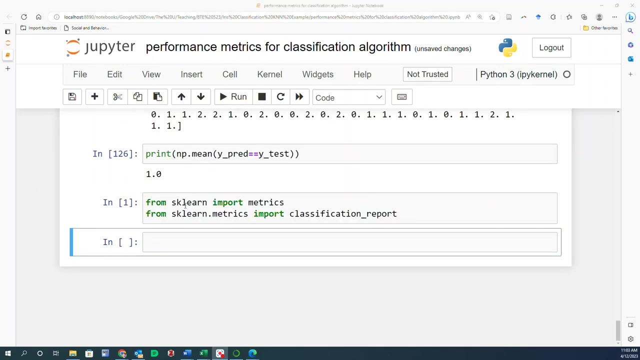 import metrics And because I'm going to, down the road, create a classification report, I'm going to say from sklearnmetrics import classification report, Classification report. All right, And just to refresh your mind, note that we did the predictions using the k-nearest neighbor algorithm. 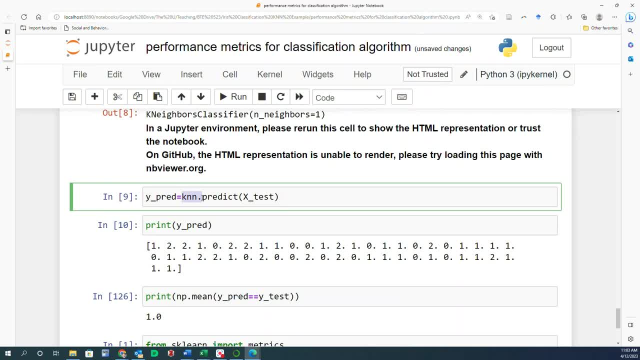 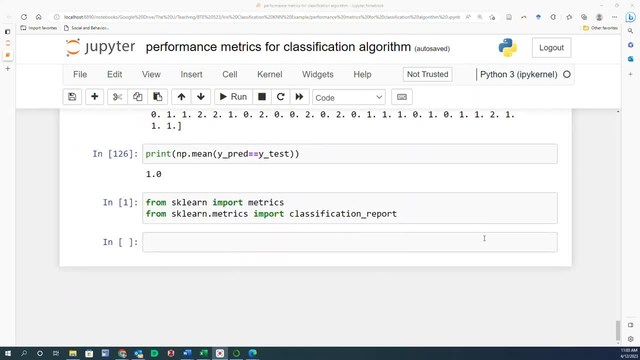 Using the KNN algorithm that we had already trained and stored the prediction in an array called y underscore prep. Now, using that, we can go ahead and actually create a confusion matrix, And to do that you'll have to type in metrics. 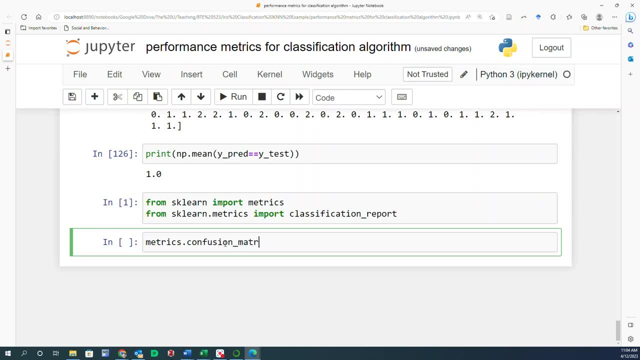 Confusion matrix. So confusion matrix is a function that's going to actually go ahead and create a function. So you can create that confusion matrix for you and it needs two inputs. The very first one is the actual classes which are stored in y test array. 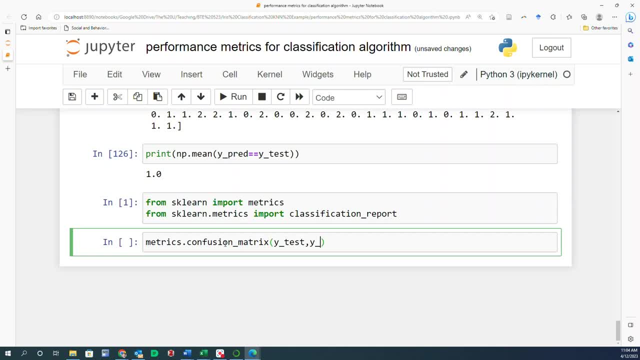 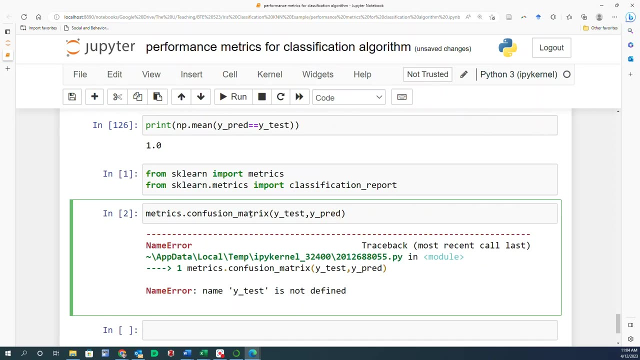 And the other one is how your model predicted the classes, which, in this case, remember, we have already put the predictions in an array called y prep, So if you do this, you will get the predictions. However, this is giving me the error because I have not run the model. 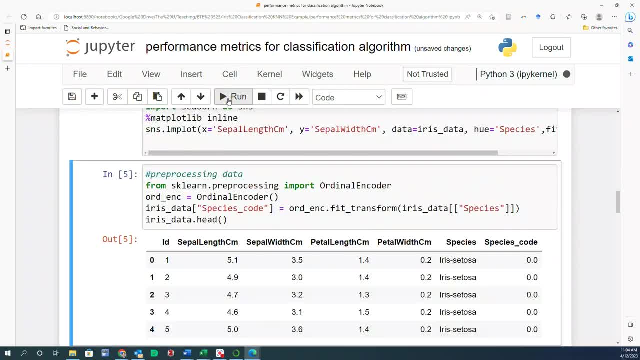 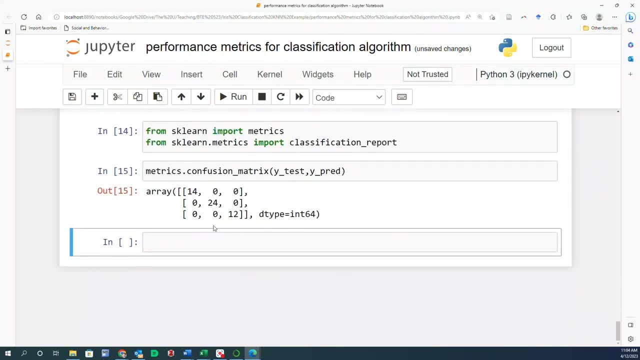 So it doesn't know what y test is. So I have to run everything from the top again And once I do that, it actually prints this confusion matrix for me. So it is fine And, as you can see, that is 14,, 24, and 12 on the diagonal and zero everywhere else, because this was 100% accurate machine learning algorithm in this case. 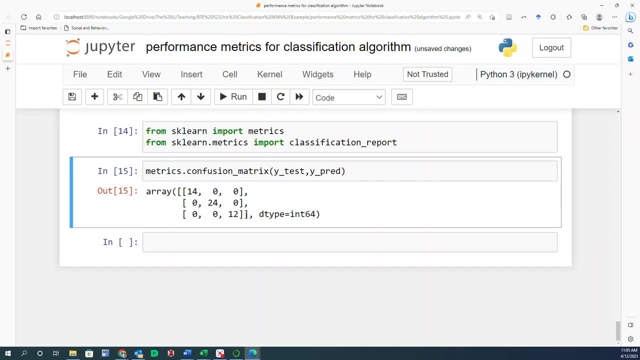 So there is nothing wrong with this confusion matrix. It is technically correct. However, what I want to do is that I want to make it much more visually appealing and informative. So to do that, I'm going to use the heat map within SNS. 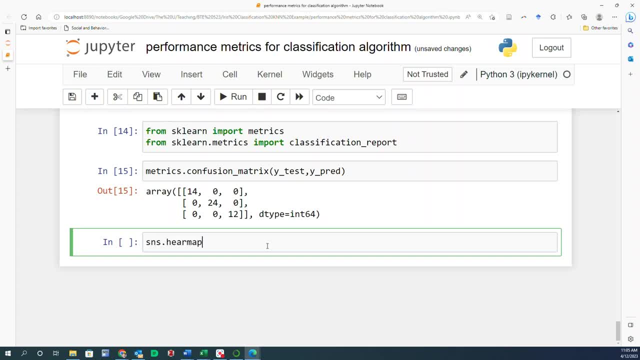 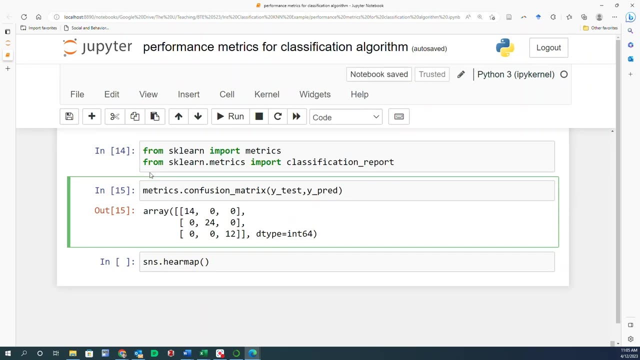 So I go ahead and type in SNSheatmap And basically what I want to do is that I want to use this and put a heat map on top of it And in order to do this, that first I'm going to put this in a data frame. So, rather than just printing the content of 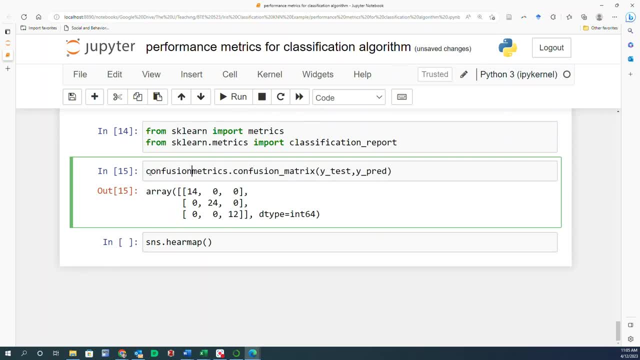 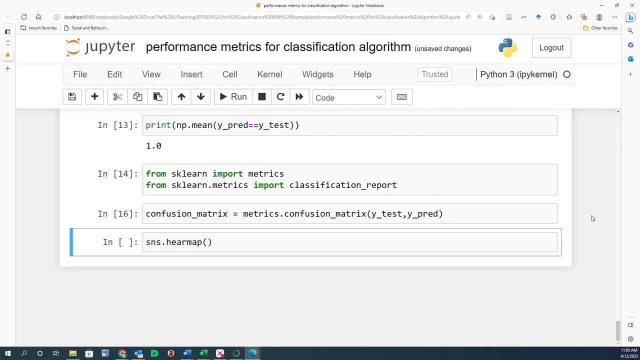 confusion matrix. I'm going to put it into a data frame that I am going to again call it confusion matrix, all right. And then once I run it, then this doesn't get printed, And then I can and say, hey, I want to create a heat map based on the values in the confusion matrix, So let's do. 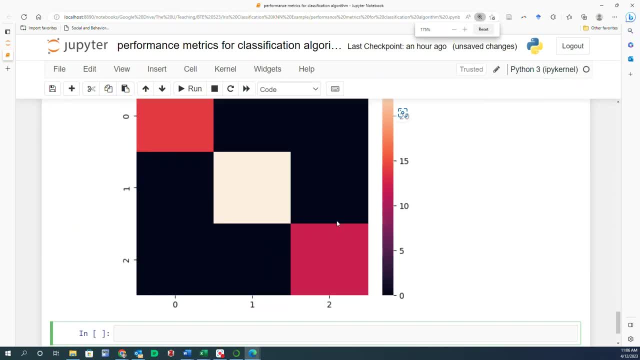 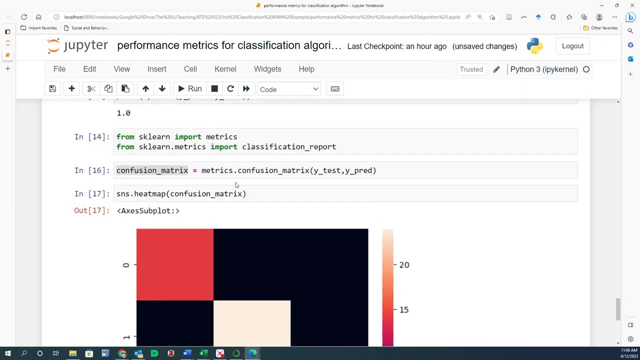 this step-by-step so that you see how it works out. So this is the heat map that it generates, and it's not really good, right, Because the colors are not nice and we don't have the values there. So let's improve it step-by-step. The very first thing that I want to do: 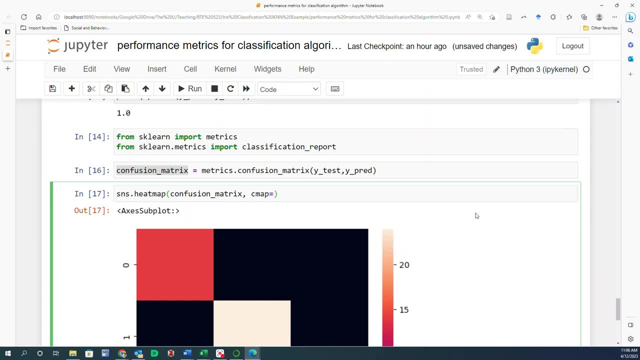 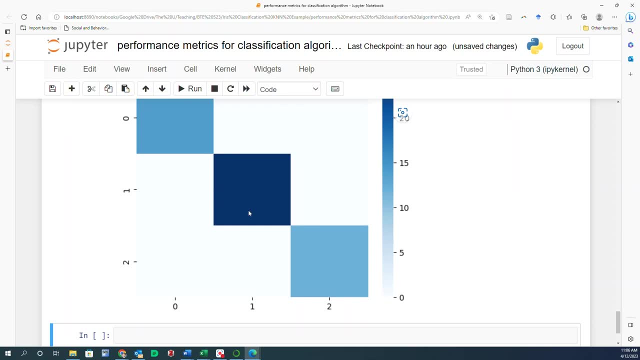 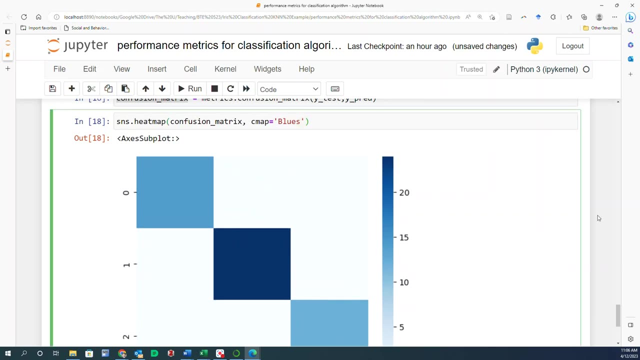 is to use the different color map, And in this particular case, I'm going to use the blues color map. So once you do that, the colors change from, say, black and red to different shades of blue, which is much nicer. The other thing that I want to do is I want to remove this color bar. So I go ahead and say: 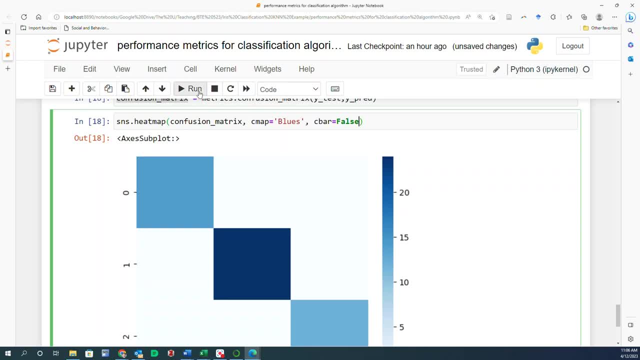 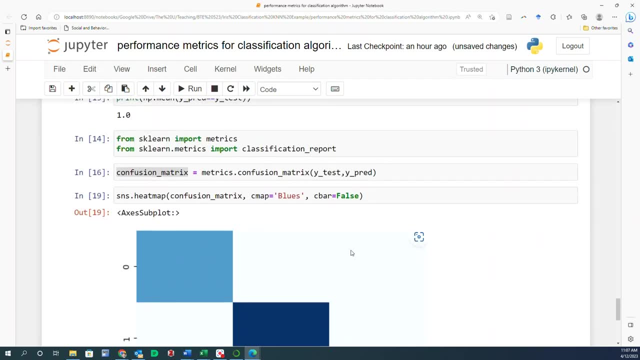 C bar is equal to false, And let me run it again for you. And you see that that color bar is removed because it was not giving us that much of an image. And then the other thing that I want to do is to actually print these values here, right To see. 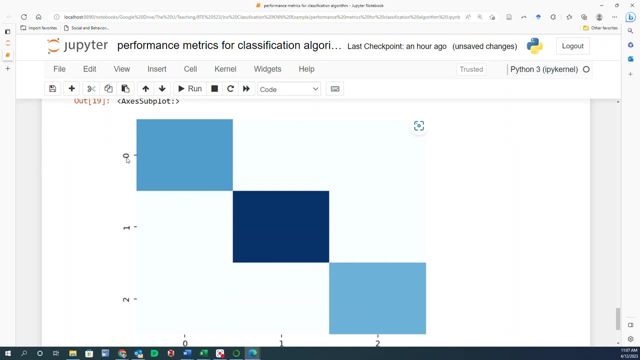 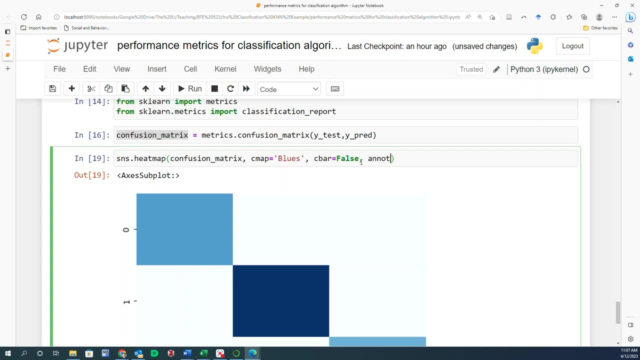 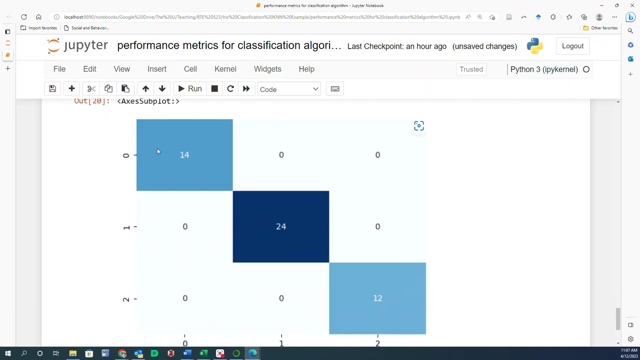 the number of instances, for example, that were actually zero and were predicted to be zero. So to do that, you can just type in annotate, or an ot is equal to true, And then it will print the values of the confusion matrix here on your heat map, right? So so far, so good, And I'm going to 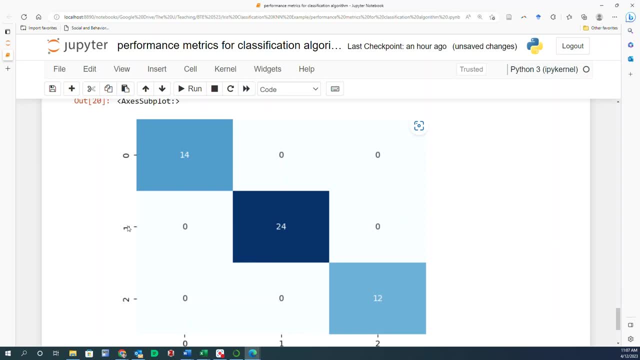 do that in the next course, Then I'm going to go ahead and go ahead and do the other things. So if I have a table that has a number in it, then I have a 0,, 1, and 2 in it. So if I want to be able to, 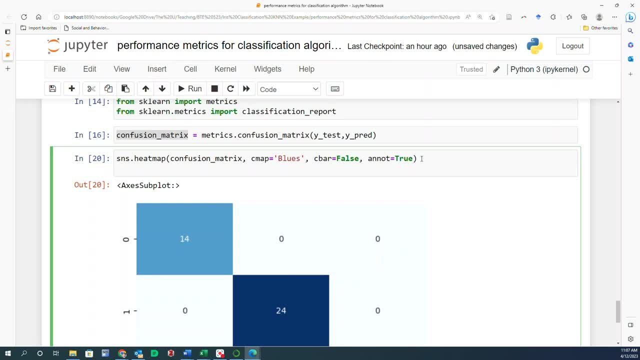 type in something like the number of instances. I can also do that. Now I want to. I wanted to do that in a bunch of different ways. One way which I'm going to do is to do that with a class of one or two, And that's the one thing that I want to do is that, rather than having zero, one and two, which were the classes of iris species, I want to type in the actual name of the iris species, and to do that I can go ahead and use the Xtics and ytics options, So I can just type in plt, Xtics. 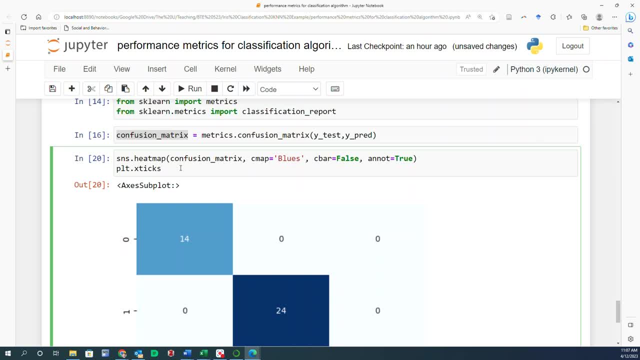 So I can just type in plt, xtics and ytics and uh go ahead and type in np dot a range, uh of three. so what does uh, np dot, uh a range does? is it's a function within numpy, and what it does is that it it creates an array that is going to have 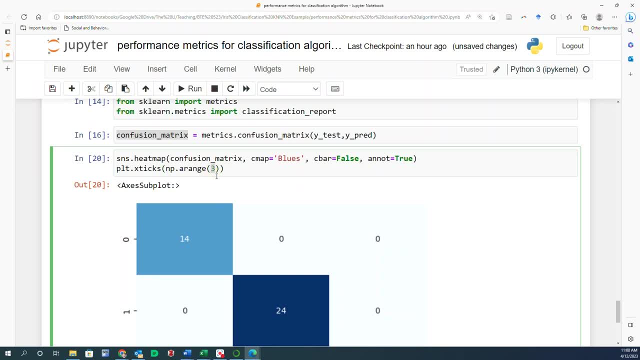 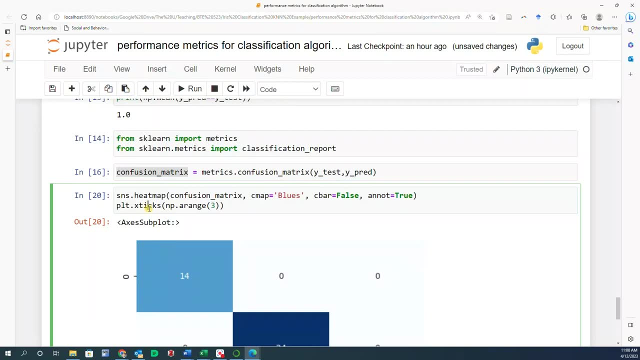 three elements, uh, and they are going to be arranged from zero, one and two, all right. so basically, i am referring to this: zero, one and two, right, so i'm going to put ticks at zero one. two positions, however: uh, i'm going to move them a little bit, so zero is going to be actually here. 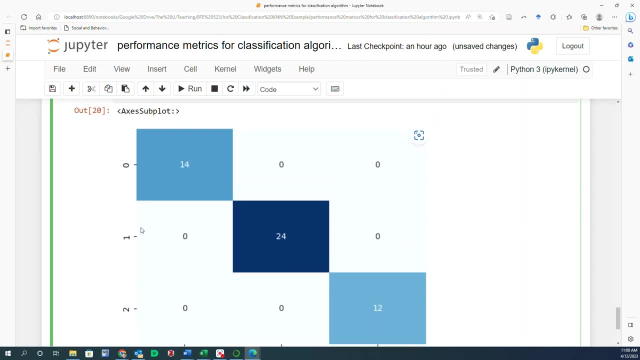 and then one is going to be here and two is going to be here, right? if i want them to be right, where you see the ticks are right now, i have to move them to the middle, and because each of them is one unit, i have to move them half a unit. 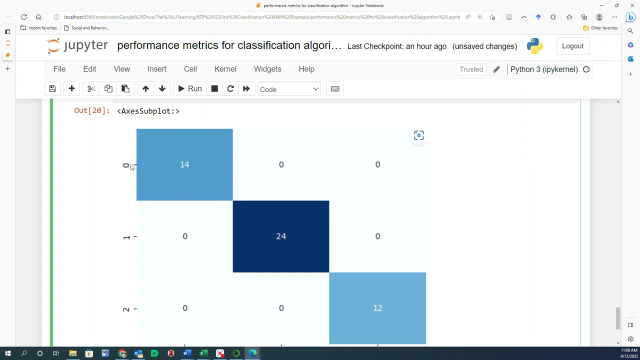 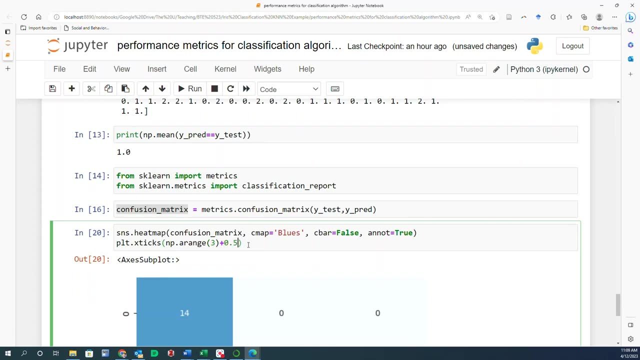 and then if i do that, rather than being here, the tick is going to come here right, exactly where i want it. that's why i'm going to say plus 0.5, and then i have to give the labels for these three ticks, and those are going to be satosa. 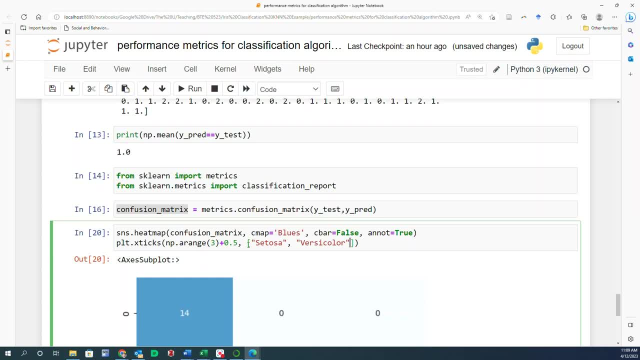 versicolor and virginica, corresponding to the class name in this dataset. all right, so that is going to create the uh labels on the text for the x-axis and i just have to change it from x to y uh in order to have the labels uh for y-axis. so 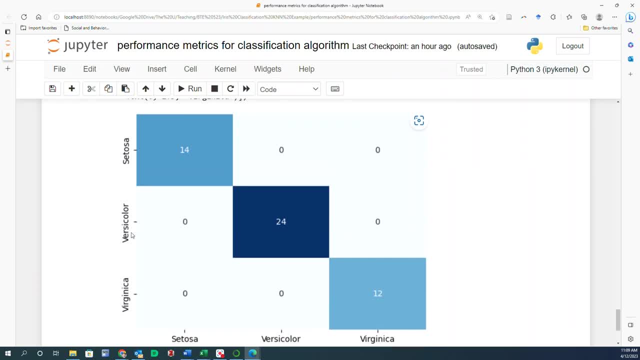 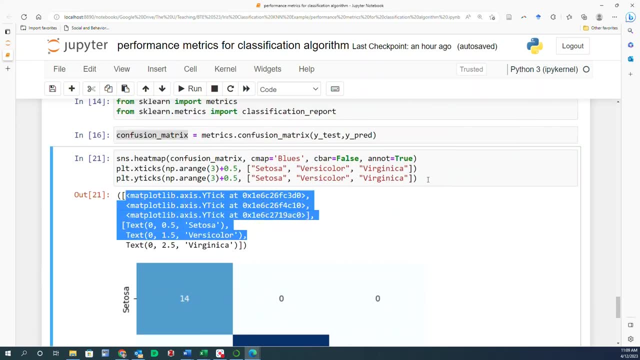 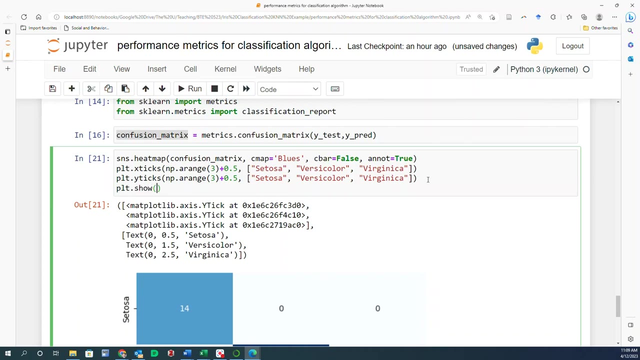 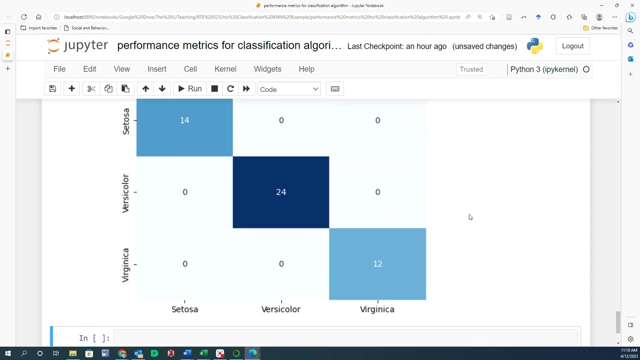 you know, you see that that zero one and two is now changed to satosa, versicolor and virginica, both on the x and y-axis, right, and if you want to get rid of this text, you can just type in plt, dot show and then it gets rid of that. now, uh, you can also, uh, enhance it a little bit and put a label for. 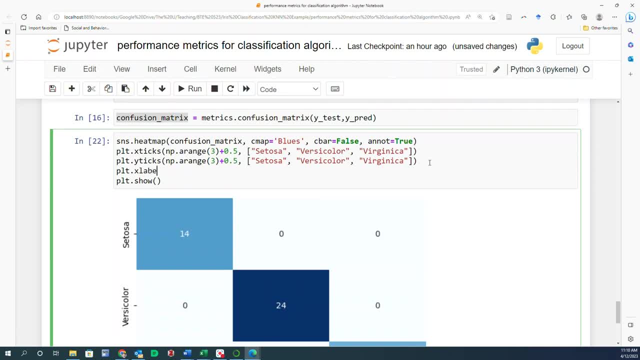 x and y-axis using the x label command. so for x label we actually have the predicted classes and for uh y label we have actual classes. all right, and once we do that, then you see that we have actual classes here and uh predicted classes here. right, very nice. 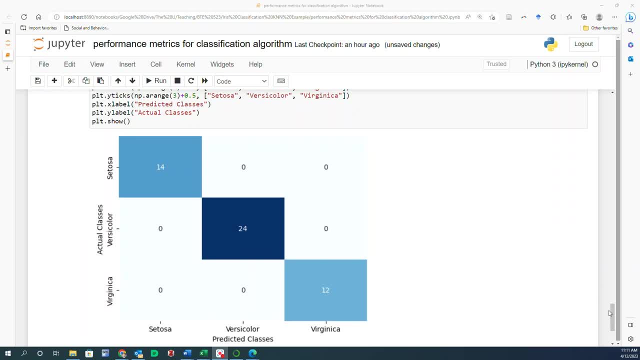 so one thing that i want to discuss here is that discuss here is that when you have a confusion matrix for a classification problem that has more than only two classes, how are you going to identify true positive, true negative, false positive and false negative? because, uh, in the video that i discussed in the theory, we only had 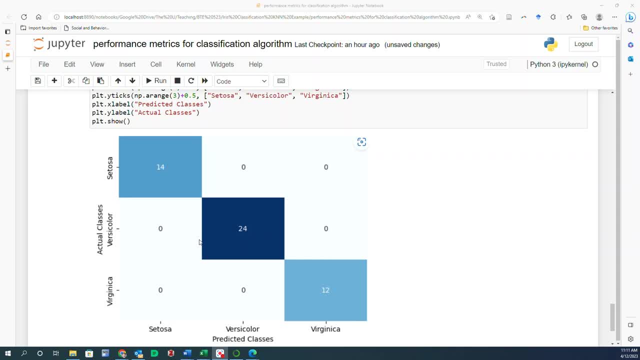 a two by two confusion, matrix, right, and it was so easy to say that, okay, this is true positive and this is true negative, and this is going to be, uh, false positive and this is going to be false negative, right, but how are you going to do that when you have more than two classes, right? 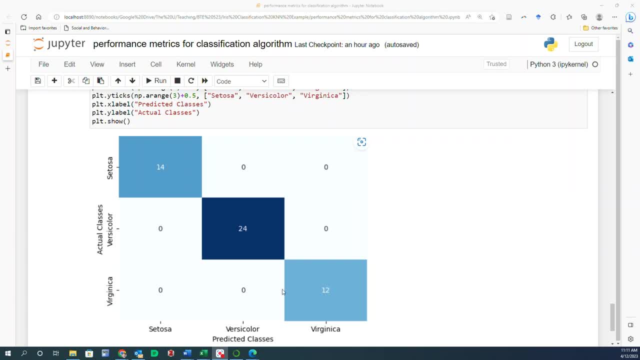 how are each of these additional cells going to be considered? uh, as true, positive, true negative, false positive and false negative. well, that is very easy, and the key thing to remember is that once you have multi-class classification problems in the confusion matrix, you have to define those. 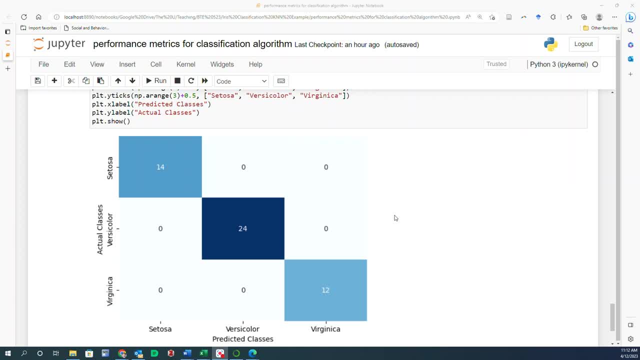 four values for each class separately. all right, so let's go over this and uh, and actually do this, and in order to uh be able to go over this concept a little bit easier, i'm going to create another matrix, another fake matrix, confusion matrix, and i'm just going to put the 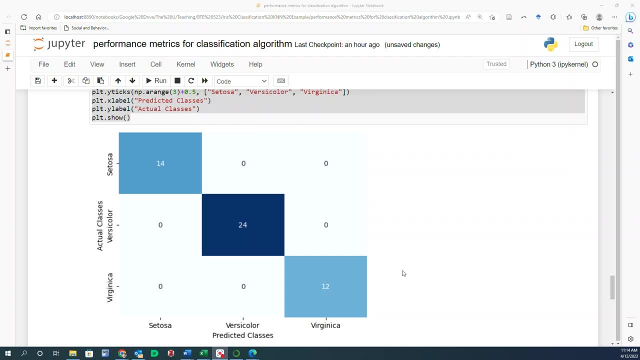 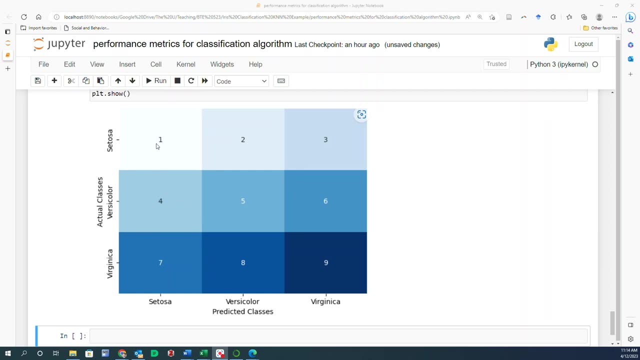 label of the cells on it, right? so this is the true confusion matrix, and what i'm going to have here is this: uh, matrix, right, that each cell is identified: cell number one, cell number two, cell number three, four, five. and i'm going to create another matrix and i'm going to create another. 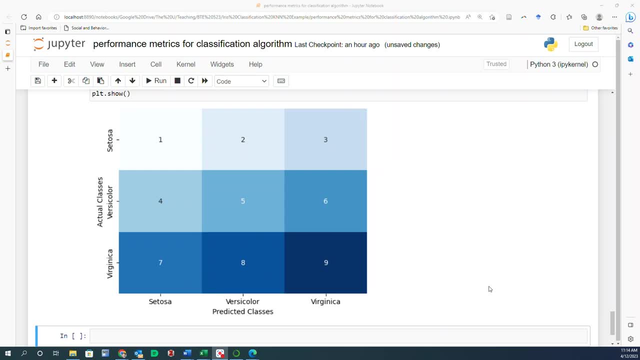 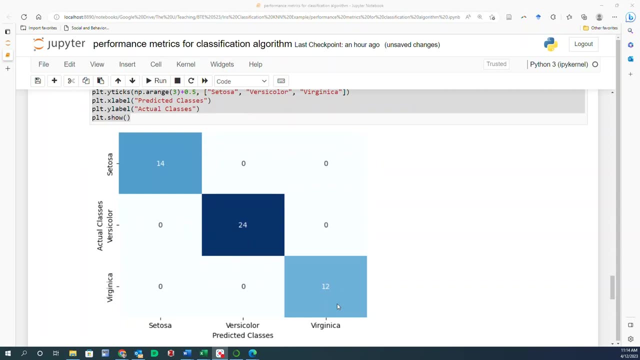 particularlys, so that as i go up and down, i'm going to do this, my zero up and down, personally, i'm going to do the same thing once again. so this is the with this default unique function: ��chest000, three areぞ is number zero and one is required to call. 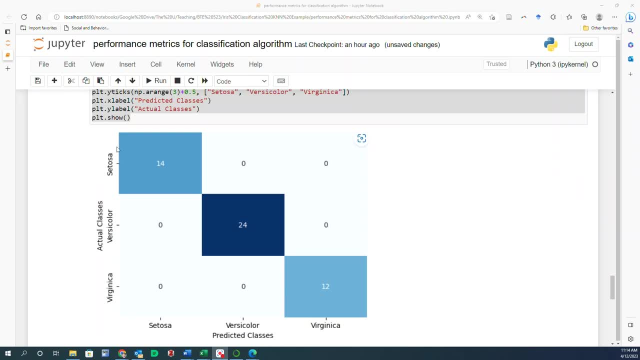 and the suffix the box with this two affair. this is the first class. so the first class is push number two, the அ- tab and the management function recommended is equal to 0.. number of instances that are actually setosa and are classified as setosa: That is going to be. 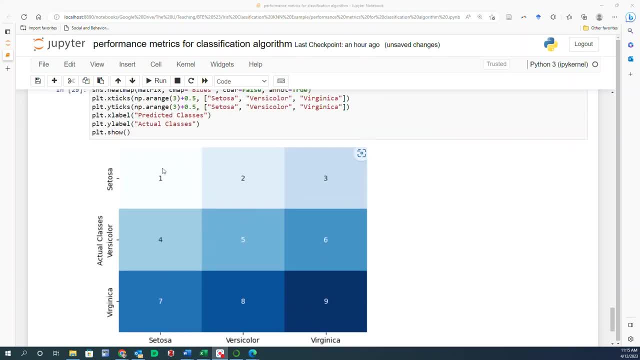 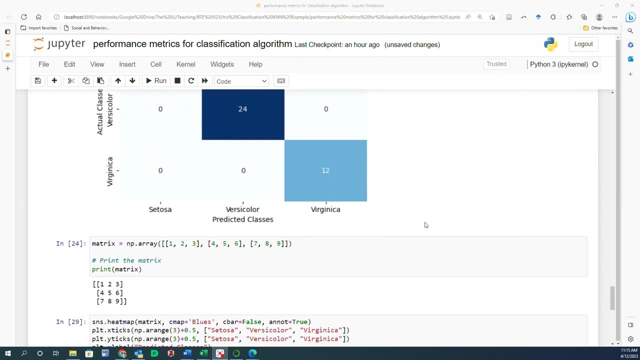 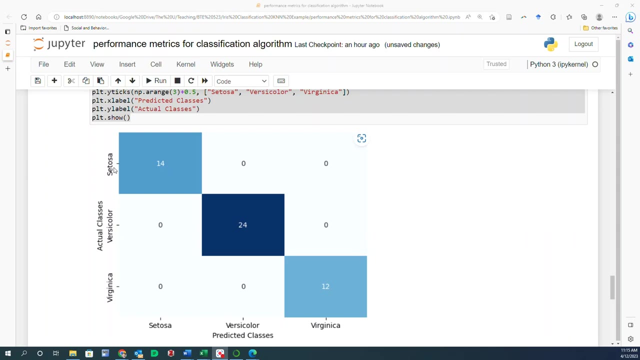 equal to 14.. In other words, when you look at this matrix, it's going to be the value in cell number one, right? So that is a true positive. Now, how about true negative? True negative with respect to setosa means that it is going to be all the instances that are not setosa. 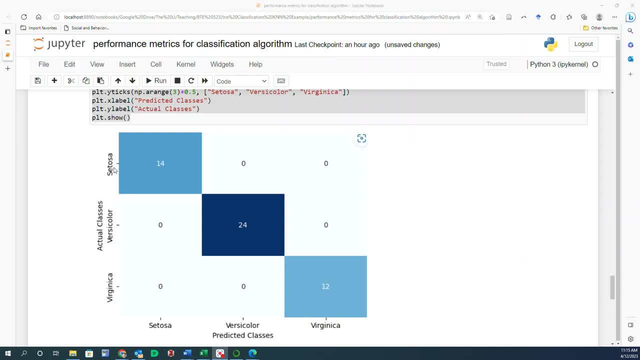 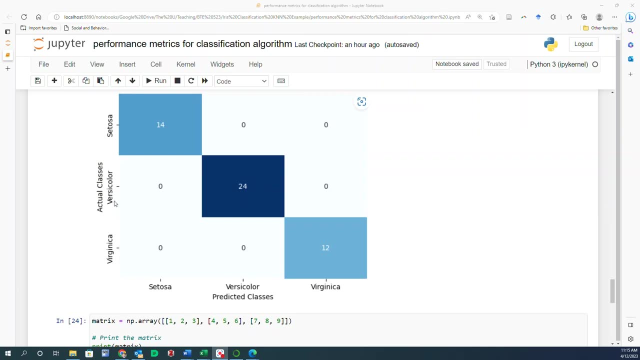 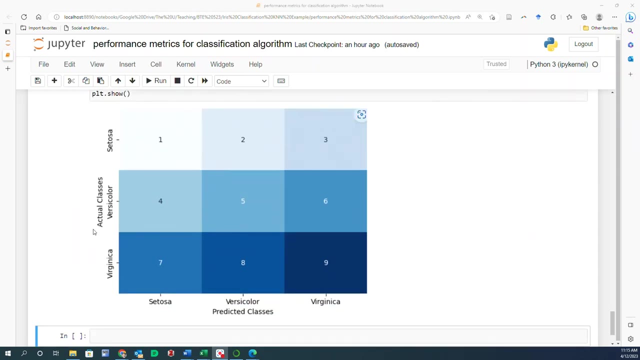 and are also not classified as setosa, right? What does it mean? It means that the classes that are actually either versicolor or virginica and are classified as something other than setosa. So if you look at this matrix again, the classes that are actually not setosa, which means that 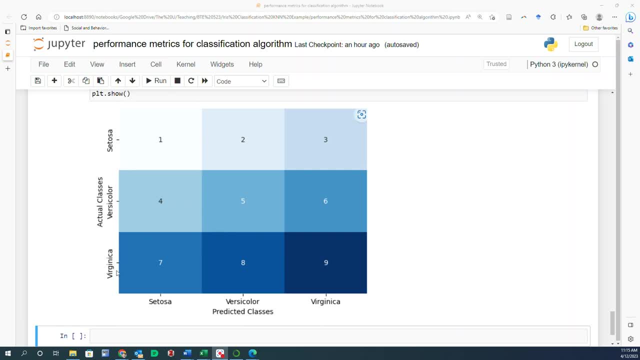 they are in row two and row three right, Versicolor and virginica. However, those species that are actually not setosa, which means that they are in row two and row three, right, Versicolor and virginica. However, those species that are actually versicolor and virginica should be classified as: 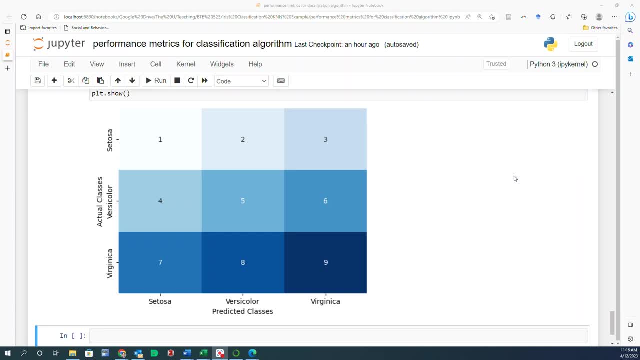 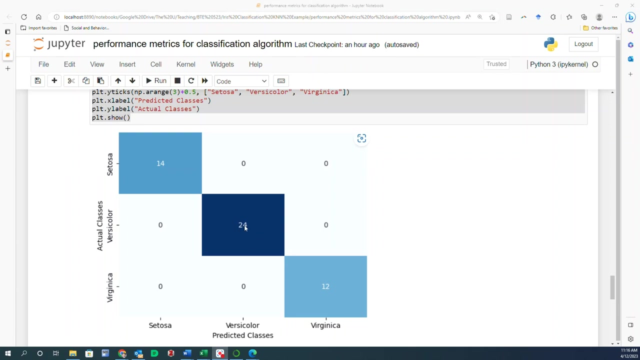 something other than setosa. So within row two and three, the first column, are the ones that say the predicted class is setosa. So anything other than that would be in cells five, six, eight and nine right. So when you look at the confusion matrix, the values for true negative will be 24 plus zero. 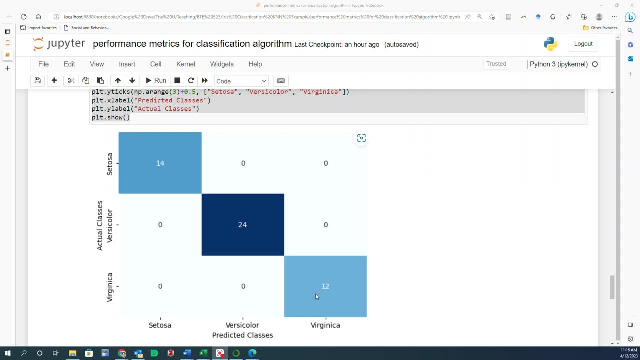 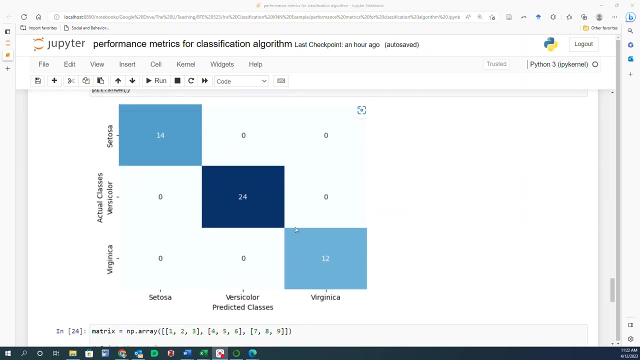 plus zero plus 12, right. In other words, it's all the instances that are actually not setosa and are also classified as anything other than setosa. How about false negatives? How are we going to define false negatives? Again, with respect to setosa, false negative means that something that 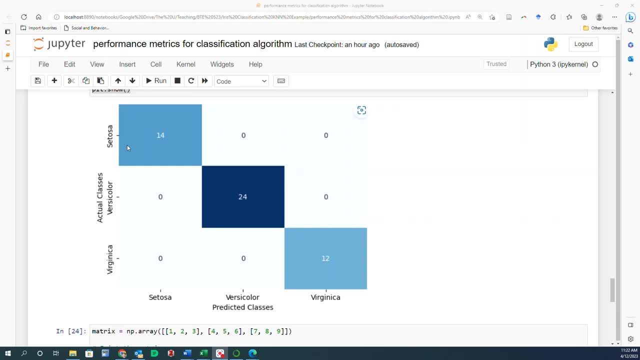 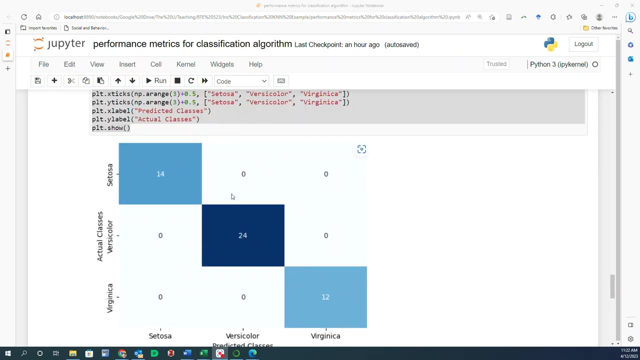 is actually setosa but is incorrectly predicted as something other than setosa. So that is going to be whatever is in this cell. and this cell specifically, cell number two and three together are going to be false negatives. Why? Because they are actually, you know, setosa, but 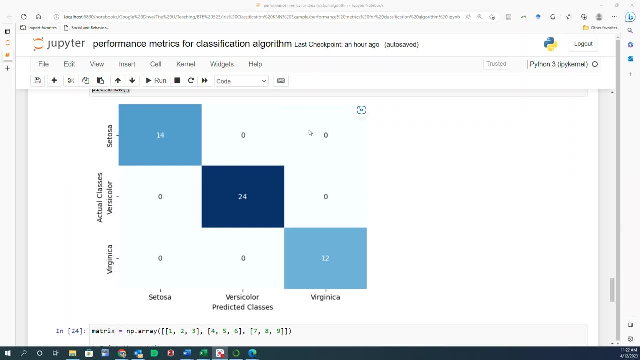 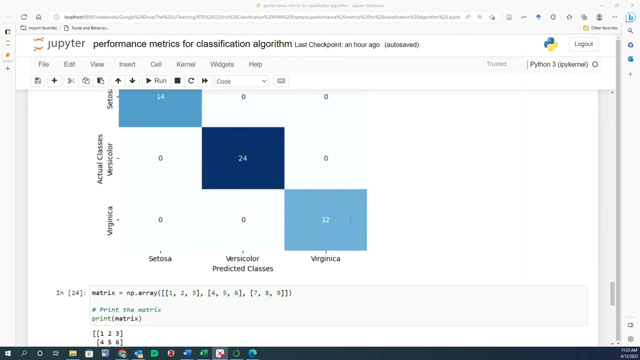 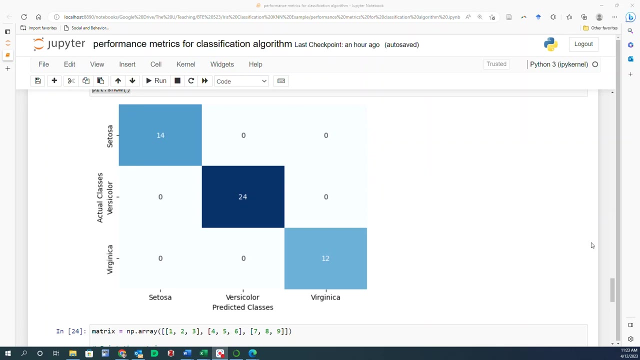 are predicted as anything other than setosa. So this is going to be our false negatives. Now, if we want to find false positives again, we have to use the same logic. What does false positive mean? It means that something that is not setosa but is incorrectly classified as setosa. So when we look 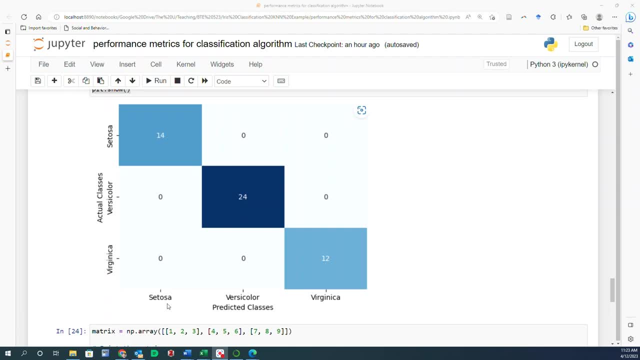 at here. you know the predicted classes for setosa are in this column. okay, So these are the instances that are predicted as setosa. right, We want the ones that are incorrect. We want the ones that are anything other than setosa, which is these two. So we want the ones that are incorrect. 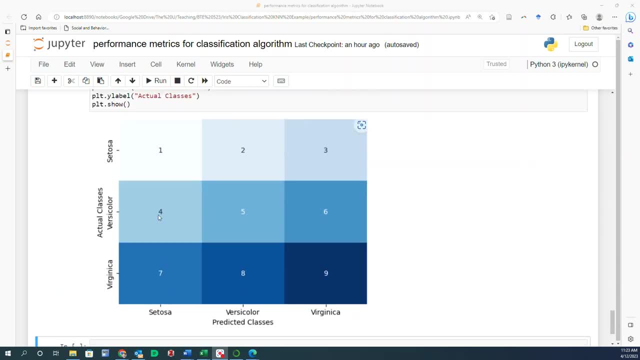 We want the ones that are predicted as setosa, which is these two cells, right? So if you look at here, it's going to be cell number four and seven. Why? Because they are predicted to be setosa. However, that prediction is incorrect And in other words, that is a false positive. So cell 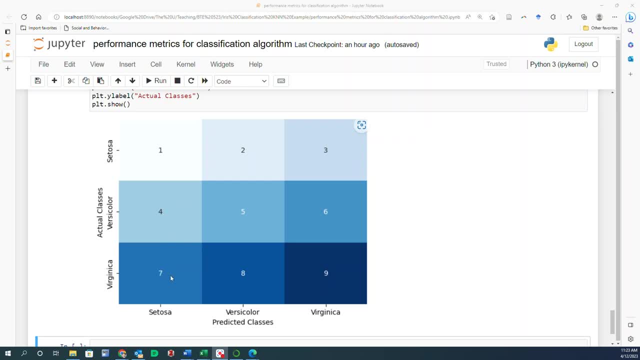 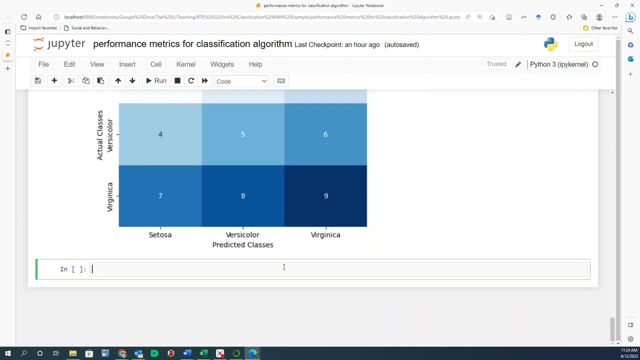 number four plus cell number seven is going to represent false positives for us. So the last thing that I want to do here is to create a classification report, And to do that you can go to the classification report, underscore report. Again, this is a function that we just imported. 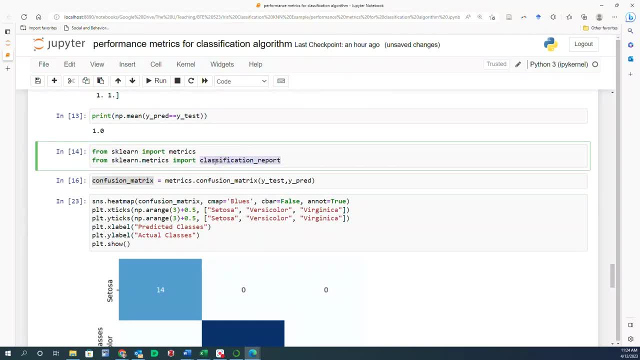 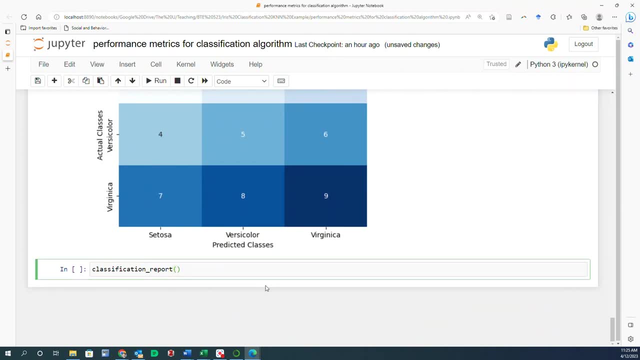 up here. Classification report is a part of the scikit-learn metrics library, So classification report creates the classification report for us And again, just like confusion matrix, it needs the two components or inputs, ytest and yprep, And the other thing that I want to give it is to put the dictionary on it, So I just type in: 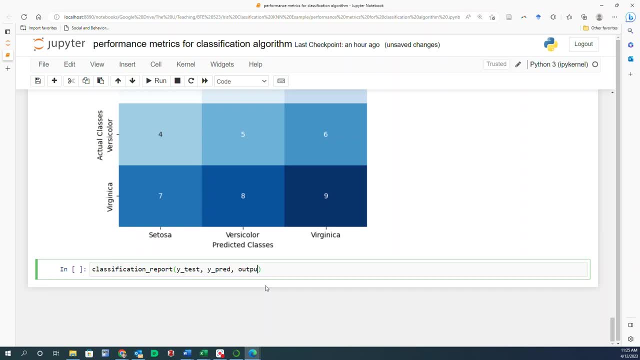 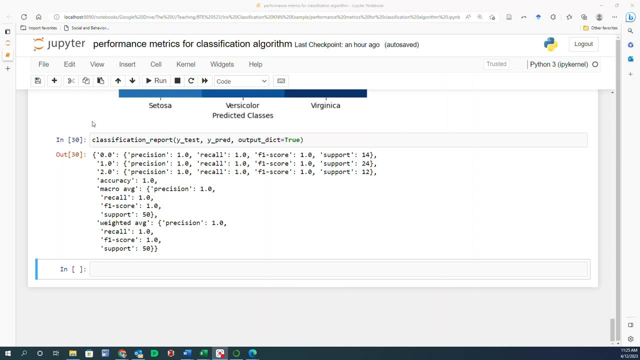 output. output underscore dict is equal to true And once you run it, you get something like this. It's not really good. What I want to do is that I'm first going to put it into a data frame. So I'm going to put it into a data frame And I'm going to put it into a data frame. 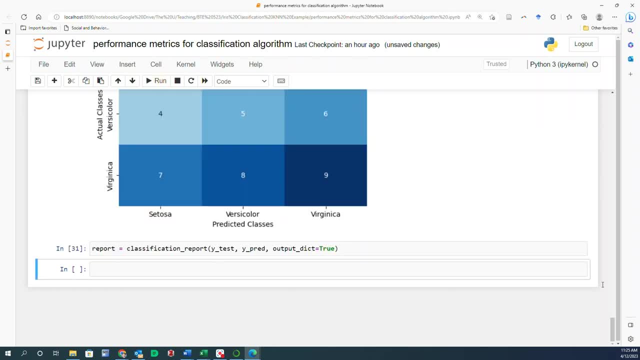 And then I just say report is equal to this. And once I have done it I go I'm going to transpose it. So I just type in final report. final report is equal to my classification report And you have to use pandas data frame here for transposing. So we are going to. 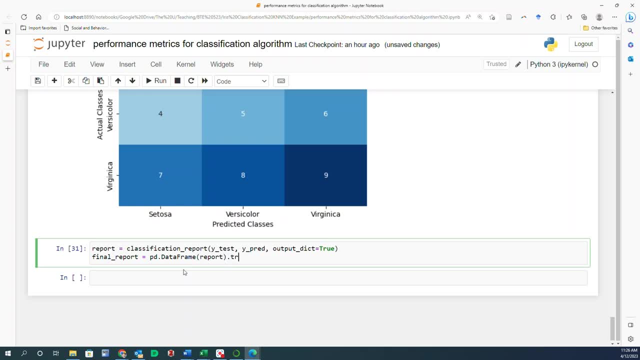 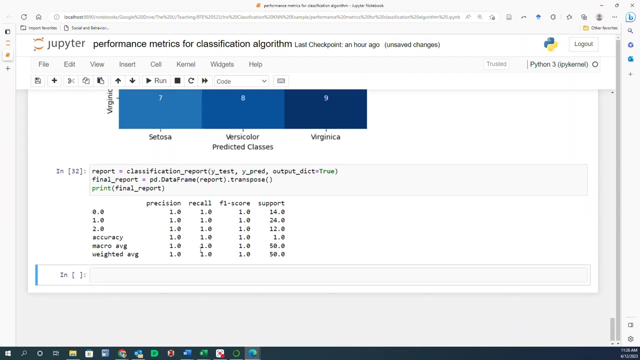 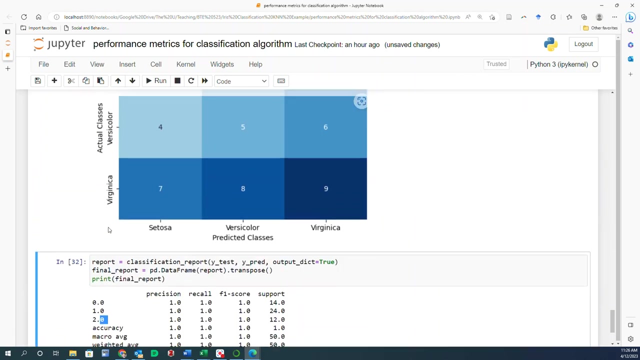 transpose this And then, once we have that, we can say print final report And we will have something like this, which is perfect, right? So here, remember that you have classification report, You have class zero one and two corresponding to Sedosa, Versicolor and Virginica, And then you 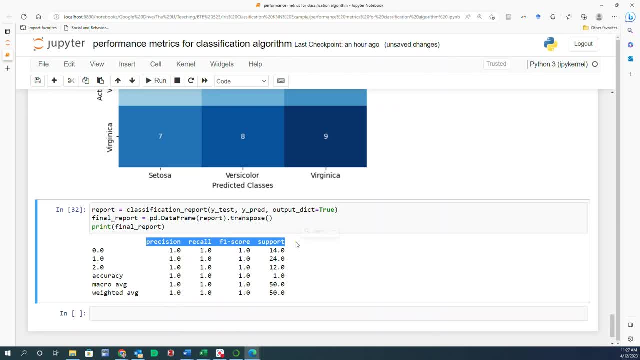 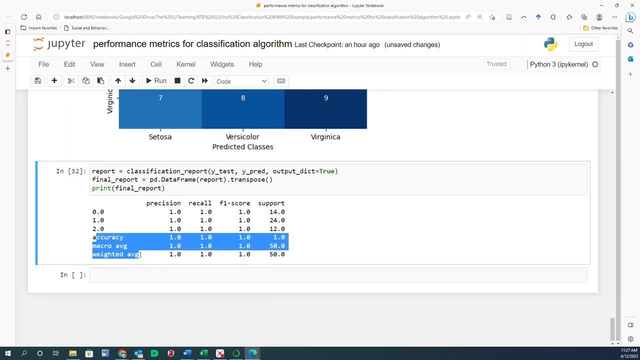 have reported precision, recall, F1 score and support for each of the classes. In addition to that, you'll have accuracy, macro average and weighted average for each class as well. Sorry, these are not for each class. These are overall right. 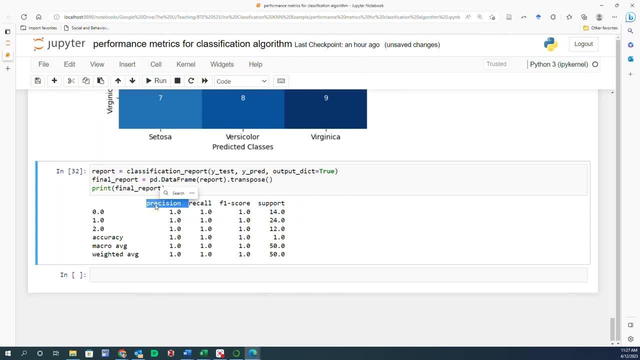 So let's go over them very briefly and discuss what they mean. The first one is precision, which, as we discussed in the previous video, is defined as the number of true positives divided by the sum of true positives and false positive. examples: right. 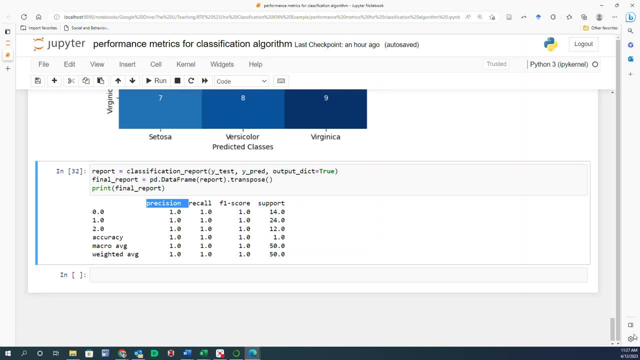 So in the example that we were working in the previous video, which was about cats and dogs, the precision is basically describing, say, of all the images that were predicted to be cats, how many are actually cats? In other words, of all the instances where your machine learning predicted a positive. 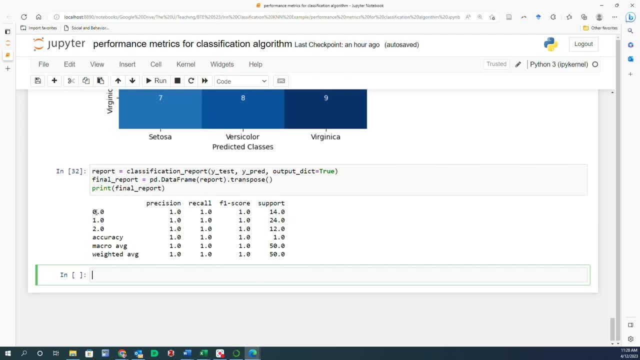 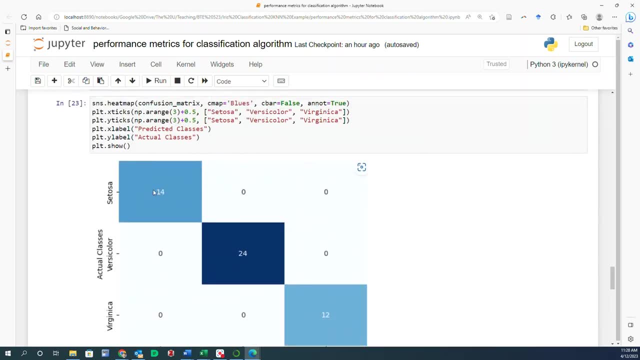 how many are actually positive, And that is with regards to the zero class, which was the Sedosa class, right? So basically here, there are 14 instances that are predicted to be positive. There are 14 instances that are predicted to be Sedosa. How many of them are correct? All of them. 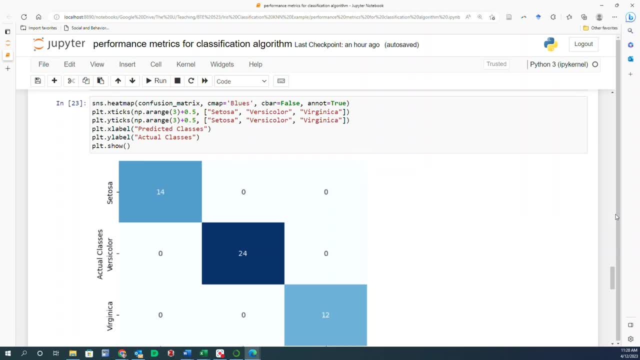 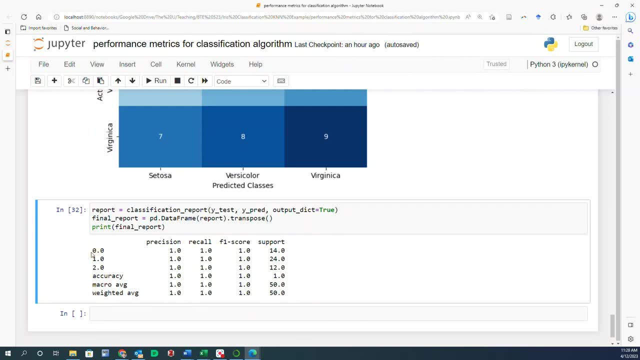 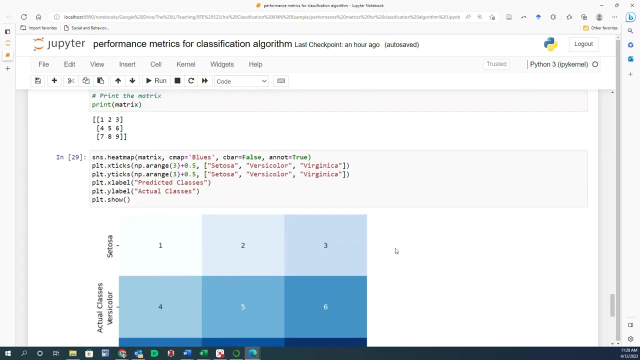 are correct, because that is all that they must be. So in this example we have a machine learning has predicted right. That's why the precision is 1 for the class of Sedosa And the same goes for class 1 and 2, right. So, in other words, of all the predictions, which is the sum of the cells? 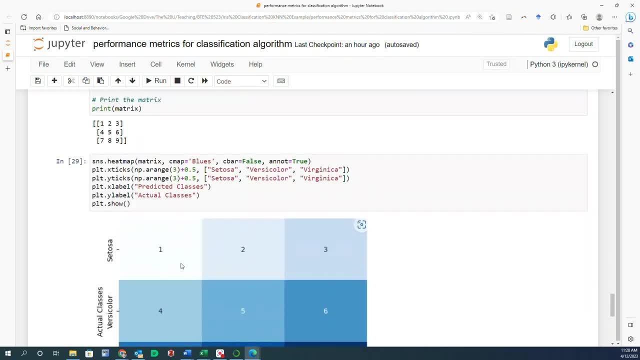 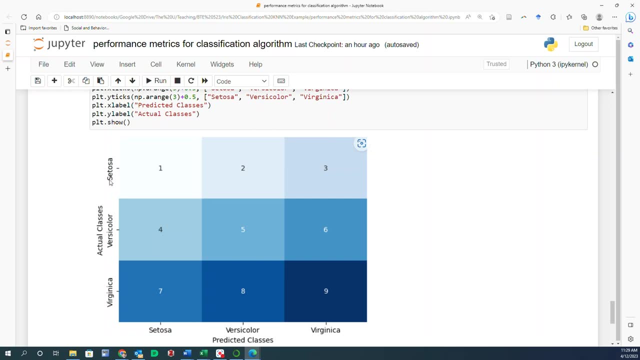 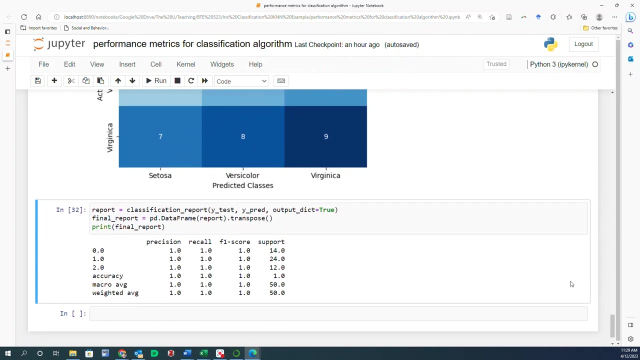 1,, 4, and 7 for Sedosa, right Of all the ones that you predicted to be Sedosa. how correct you were right. In what percentage of instance you were correct, and that is going to be 100% for precision. 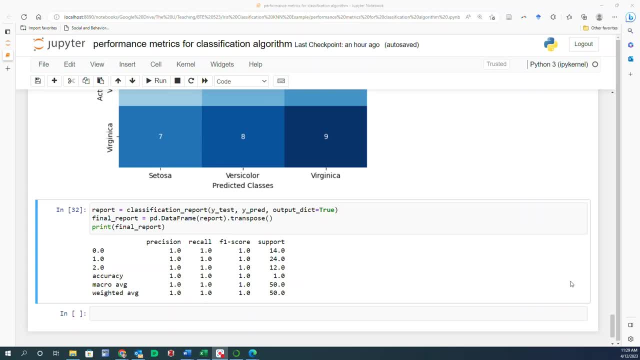 Recall, on the other hand, is defined as the number of true positives divided by the sum of the true positives and false negatives. In other words, it's asking: out of all the real true positives that are existing in the data, how many could you find? 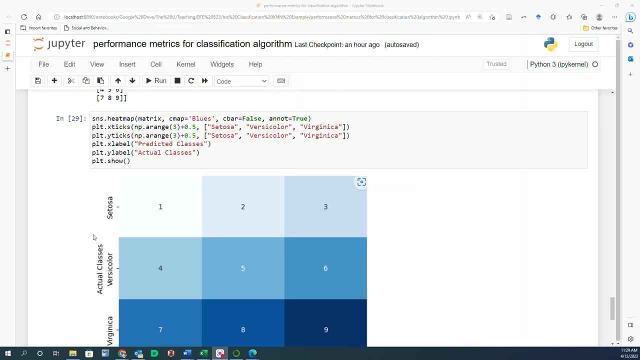 right. So, basically, when you look at here the actual class and after identifying the verse 1, you're going to be asked what percentage that are with type Labrador. is that the real RealB Around? It will then start to be 1.. So if you ask us what your awareness is, there are different counts. 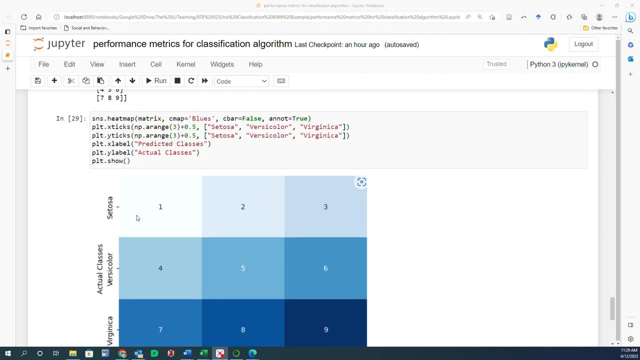 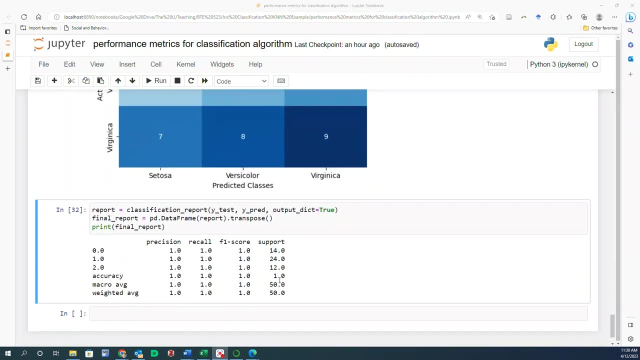 for a легко. As I said we originally, You know, for sap. let me enough value. So we underneath整 here we haverée. besides, per you can see how there is a limit of when between them and 3000.. This is why we white. So this is. 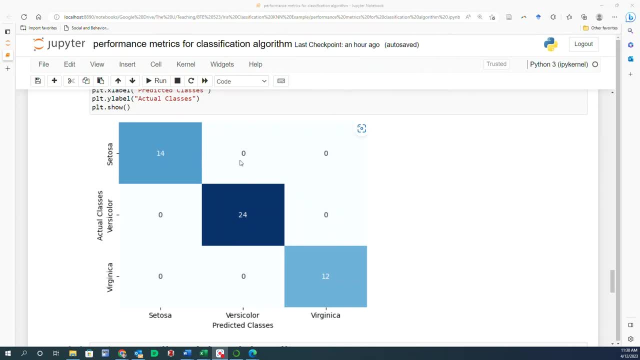 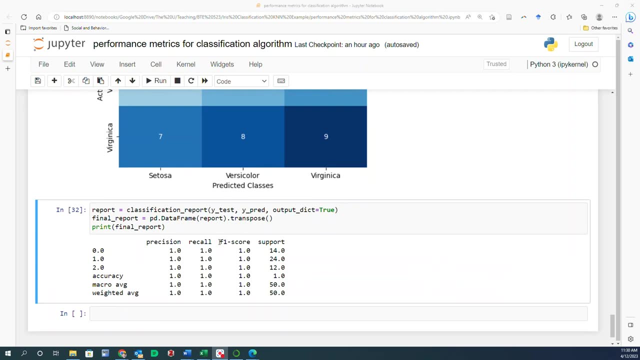 itはい A little bit of intensity here. you know That's how devaming about analytical classes for SadAttack hospital. So, and the cells out of 14 plus 0 plus 0, right. The other thing is the F-bond score. 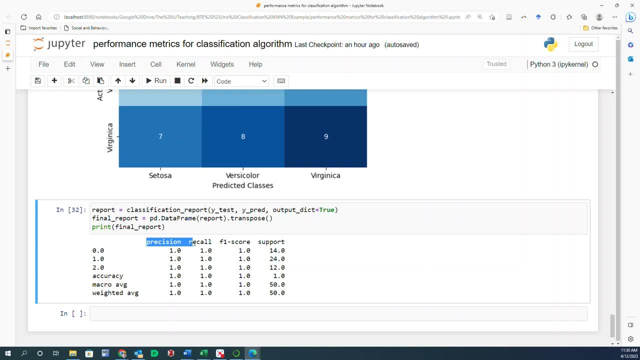 F-bond score is an average of precision and recall, And it's a really good metric when the data set that you have is imbalanced, meaning that there are more instances of one class than the other right. This is not the case here, but if it was, the accuracy may not be a good metric. 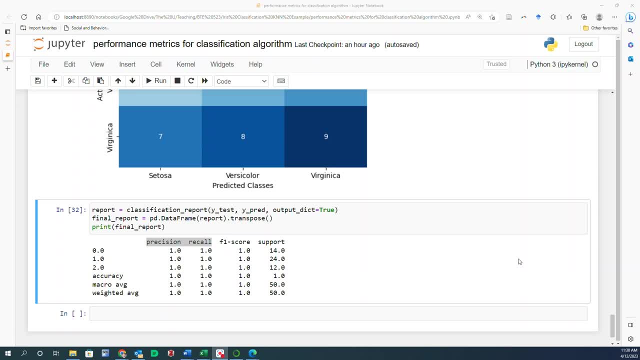 and therefore a better metric would be an F-bond score. Finally, support indicates the number of instances within each class in the data set, regardless of how well you predicted them. So it basically says that there are 14 of class 0,, 24 of class 1,. 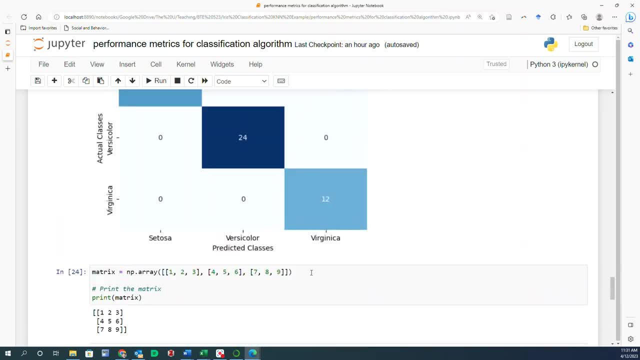 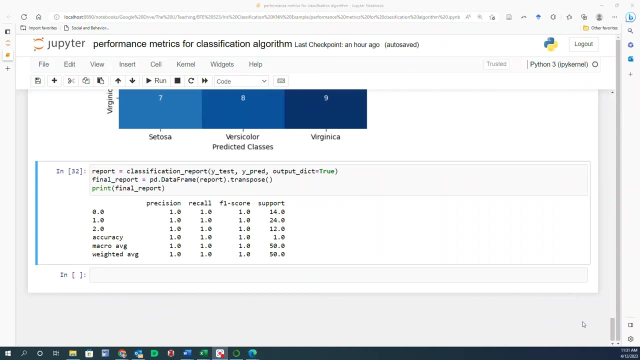 and 12 of class 2.. So, basically, how many instances of each class exist in your testing data set? Similarly, you have accuracy calculated for each class, as we've described before in the video. That is going to be the ratio of true positives and true negatives.